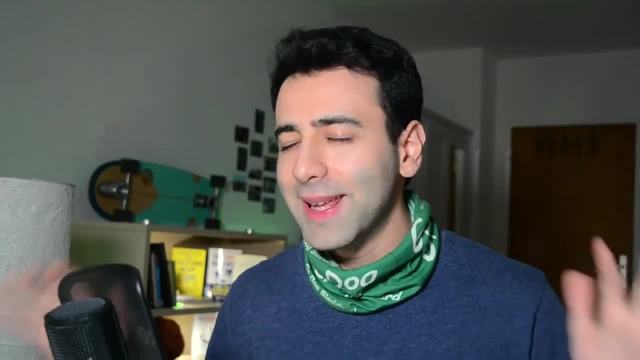 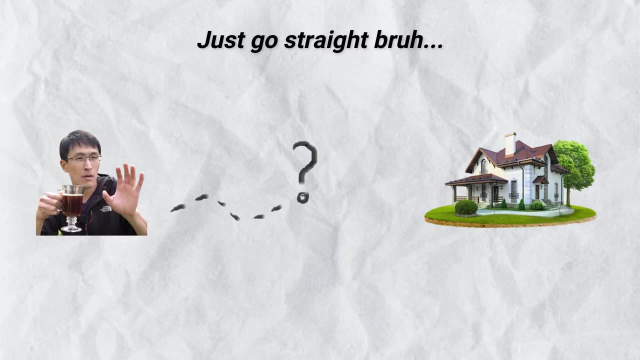 be much clearer once we see the code, I promise. But for now, imagine a friend is coming over and they don't know where you live. The imperative approach would be giving your friend detailed directions for a specific route to your place. The declarative approach would just be giving your friend an address, a map and letting 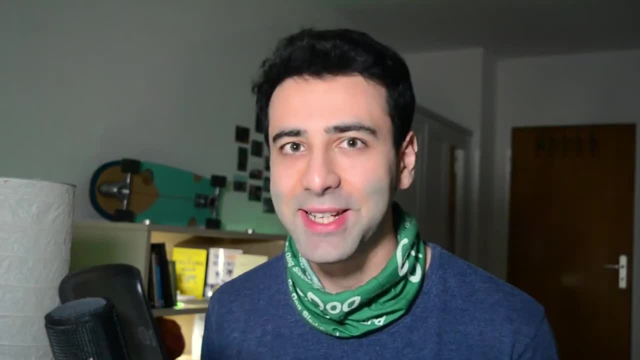 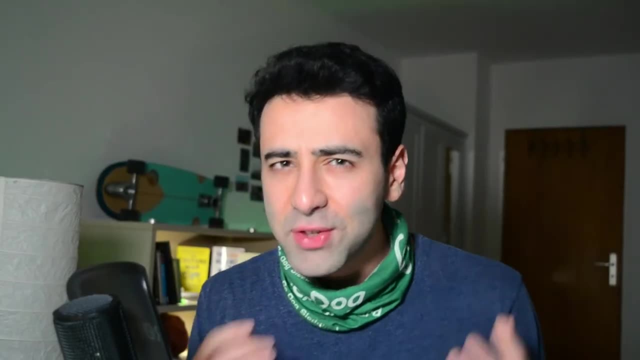 decide how to get to your place on their own. Just as a side note, if you want your friend to get to your place as soon as possible, make sure you smash the like button. this will help out tremendously. But here's the most important part. 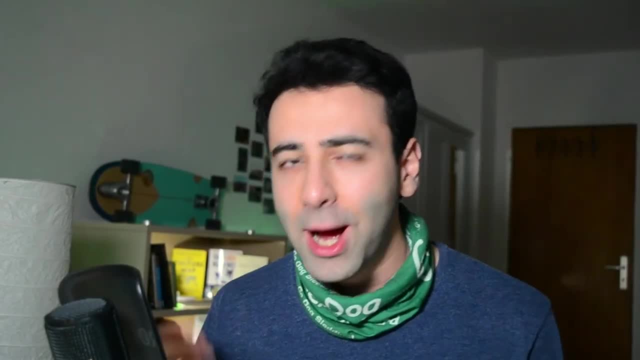 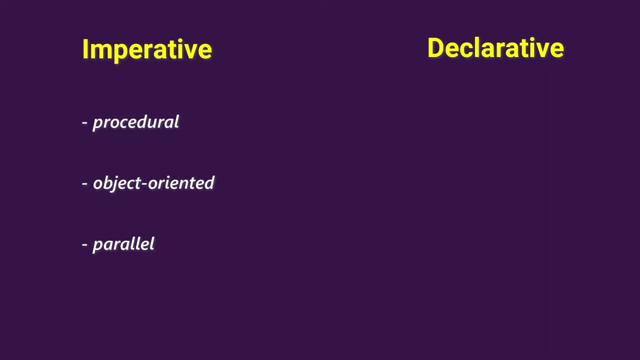 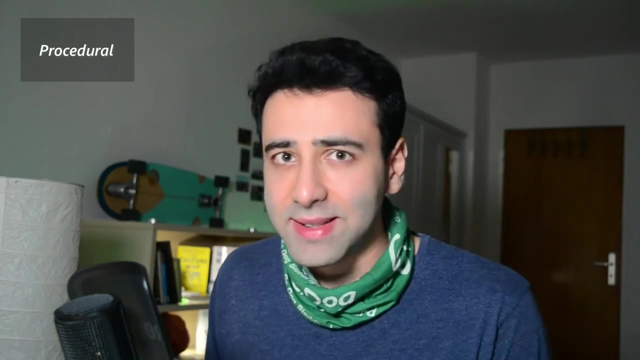 Each category has a subcategory which will define how exactly your code is going to look like. For example, imperative category is divided into procedural, object-oriented and parallel paradigms. First, the procedural one. The funny thing about it is that the idea behind it is the same as its parent, that we 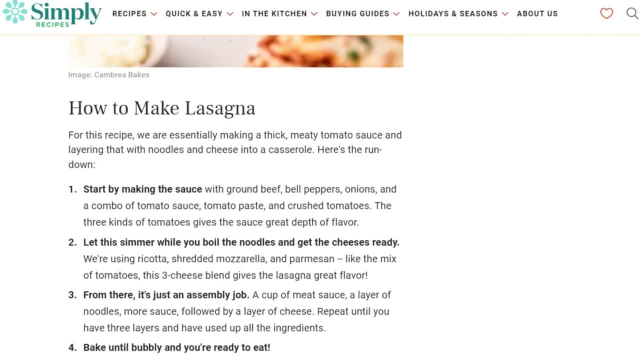 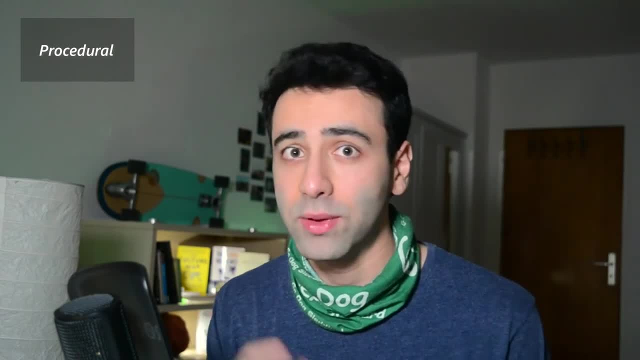 already discussed. It's essentially like a recipe that a computer can follow. The code can be reused in different parts of the program, given that you nicely separate some chunks and put them into functions. Another benefit is that it's simple to read and understand. 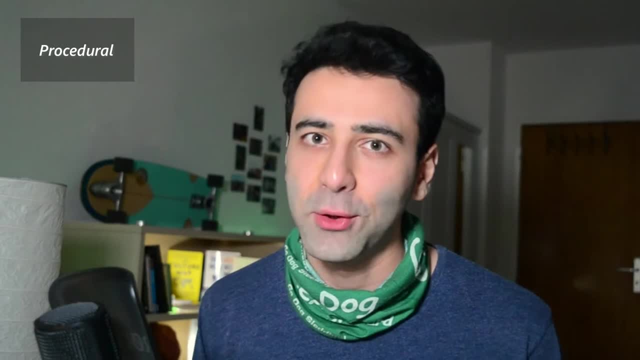 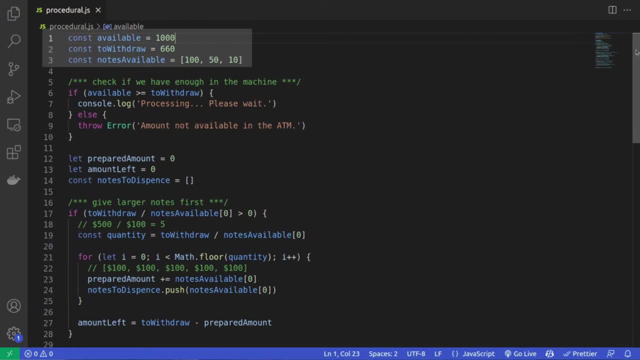 Although, when dealing with complex problems, there's a risk that you can end up with a huge volume of code, We start off by declaring the variables that the ATM has already built in. Let's start with the code. At the end we get a few more variables. 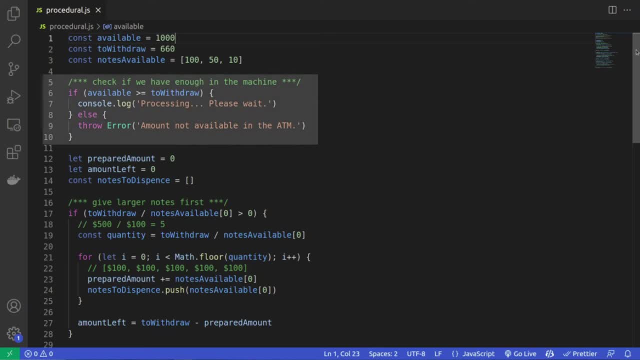 We can start by checking if the ATM has already built in some new code- that's why we call it a custom code- or received from a customer, and jump right into the next step, which is checking whether the requested amount is already available at the moment. 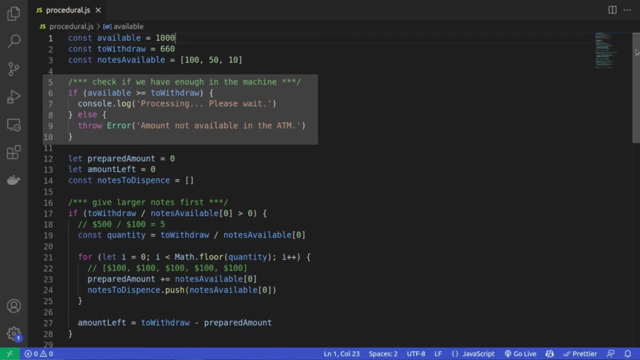 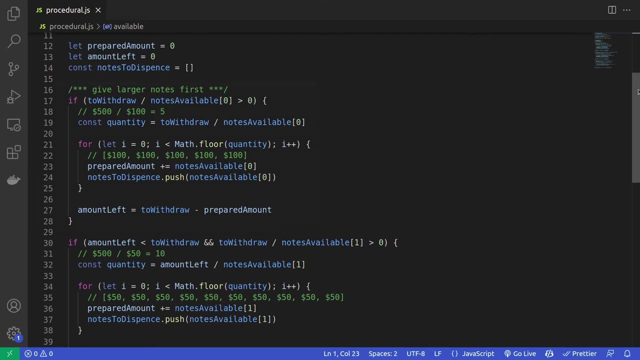 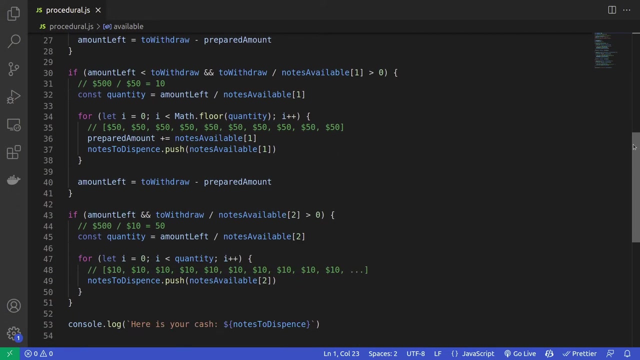 If so, we will proceed. otherwise we throw an error by explaining what happened. Then we are calculating how many nodes we need to dispense, and start off with larger nodes, as every ATM does, of course, which is quite annoying. We then get to smaller nodes by checking whether we have the needed amount every time, and 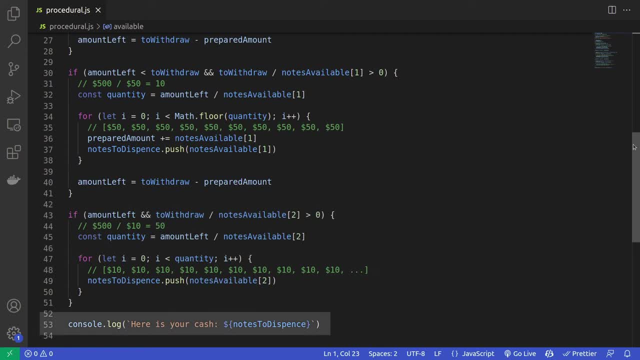 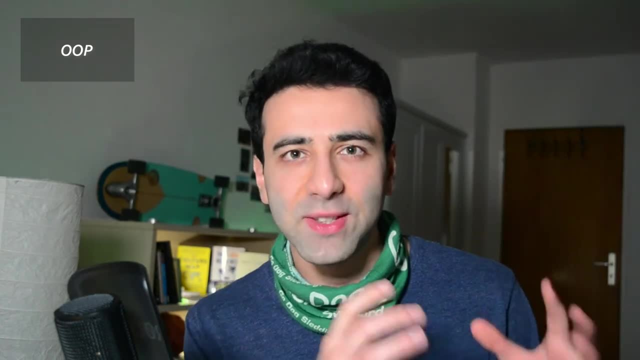 at the end we get the value of the code. give the customer a list of nodes to dispense. Now the object-oriented subcategory, or rather object-oriented programming, is different in a way that it's based on an idea that code can be broken down into classes that 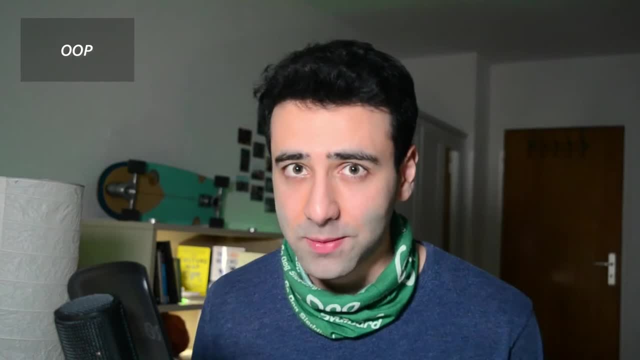 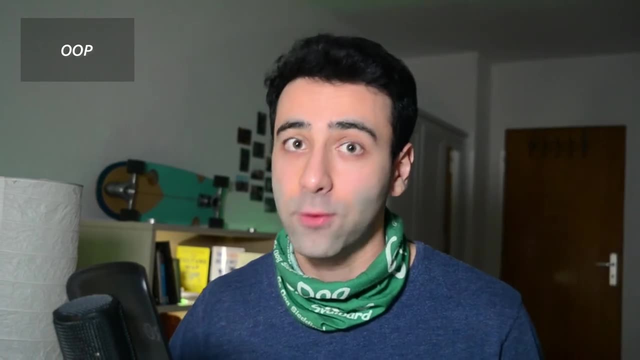 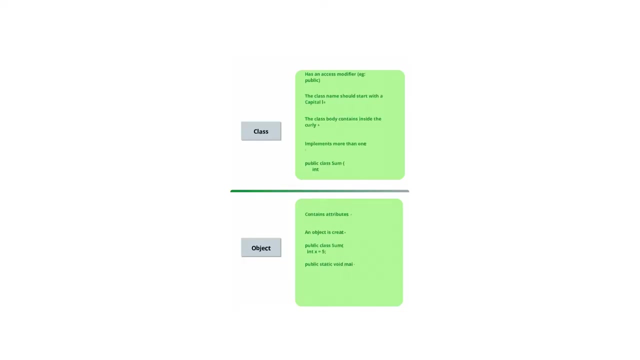 have different properties and can perform different actions. Objects created from those classes are meant to communicate with each other and inherit methods and properties from each other. The reason why OOP is so famous is because it mimics our real-world view of objects, making it easy to grasp. 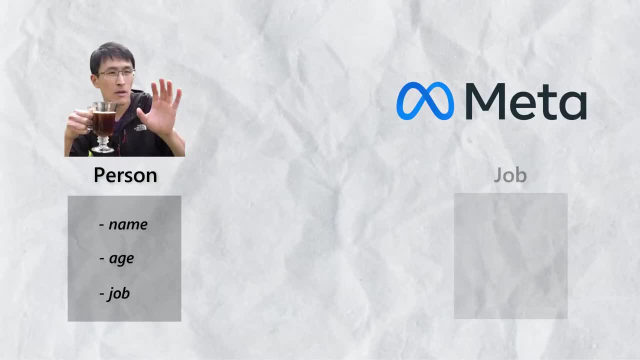 Class Person has a name, age and job properties. Class Job has a work method. An object created from a Person class can call a function of a Job class to make some money Using OOP. in our ATM example would look something like this: 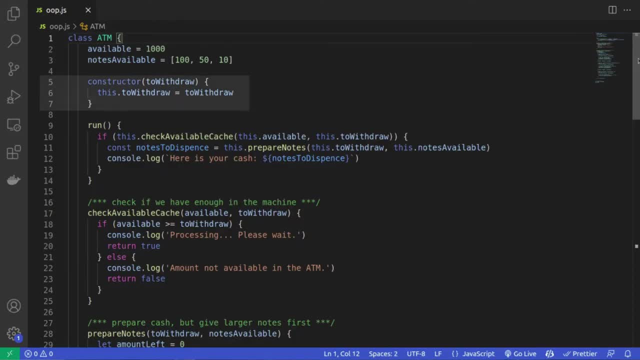 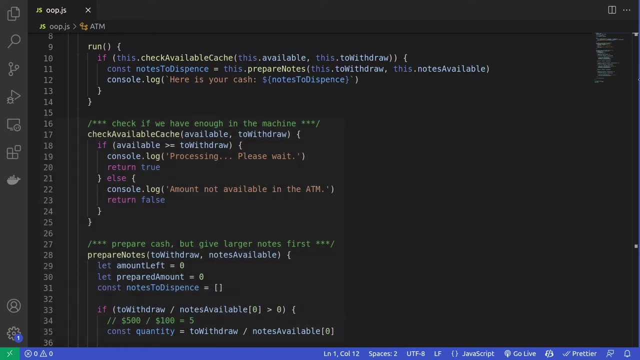 We have one ATM class that has a constructor that receives a desired amount to withdraw from a customer. Then we have the same functions we had before, but as class methods now, and we have a new run method which kicks off the whole process by calling all other methods. 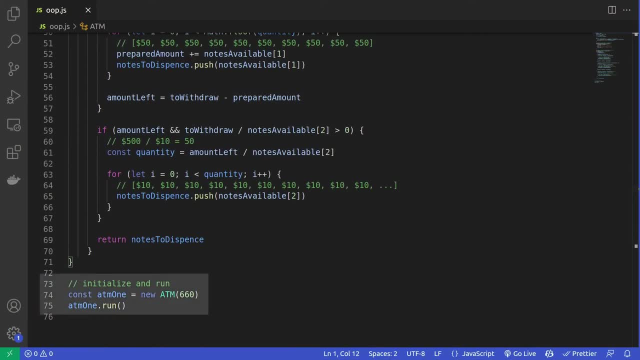 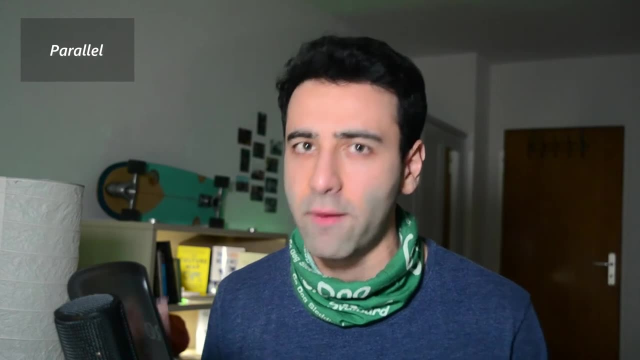 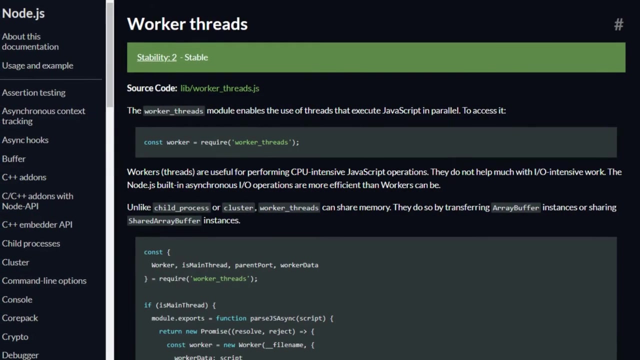 We create a new instance of the ATM here and call the run method. The last imperative subcategory is parallel processing, which many would argue does not exist in JavaScript. In fact, that's no longer true With the introduction of web workers in browsers and worker threads in Nodejs. there is now 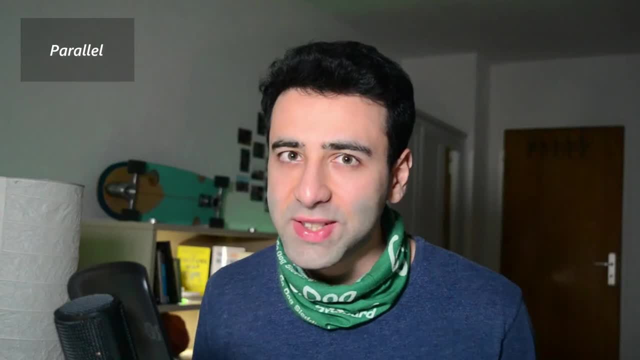 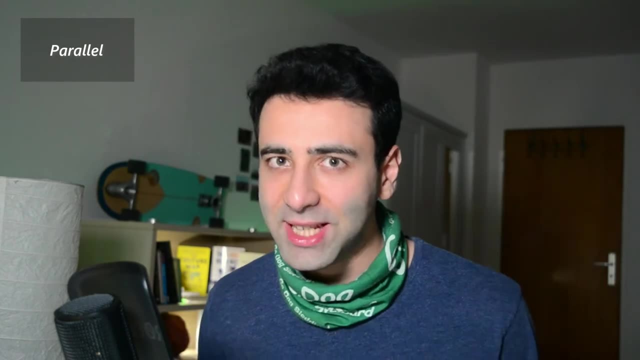 a real way to do parallel programming. in JavaScript Workers are only useful in CPU-intensive operations, which means we won't be using it for our ATM example. Essentially, the way it works in a browser is that every tab you open gets assigned a separate thread that executes the code. 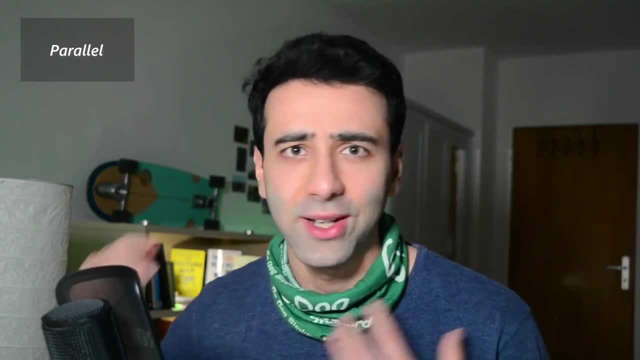 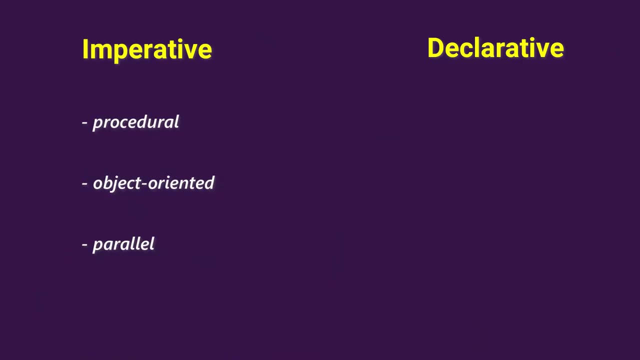 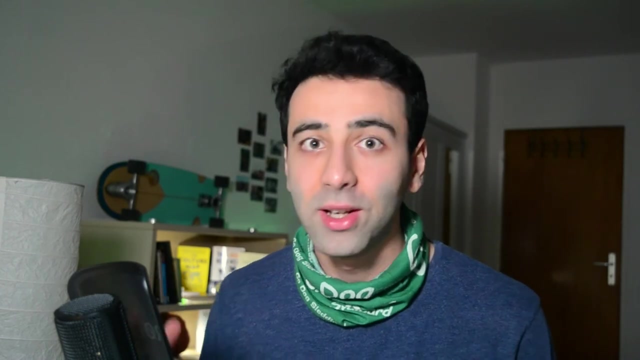 But with web workers, you can create arbitrary threads for a single tab. The same principle works in Nodejs: you simply require a new worker thread. Now that we're done with the imperative side, let's talk about the declarative side. The declarative approach includes functional programming, logic programming and an auxiliary. 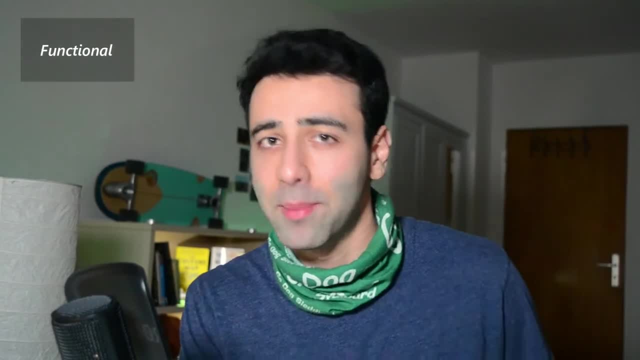 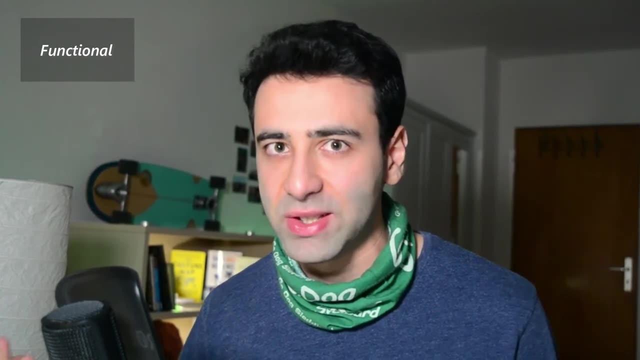 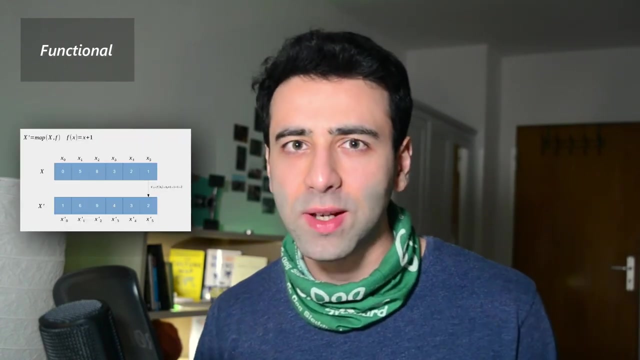 data-driven programming. Functional programming has its roots in mathematics and is somewhat a language-independent paradigm, which means you can implement it in many programming languages. as long as you try hard enough, You can basically write functions that carry out every types of tasks without using a global. state or mutating any global values. That's where the immutability comes in. Functional programming also tries to avoid things like loops and instead relies on recursion. This paradigm generally reduces complexity, but in some cases it can be really difficult to scale with it. 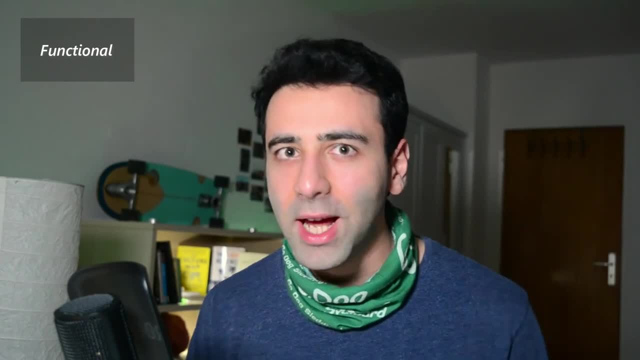 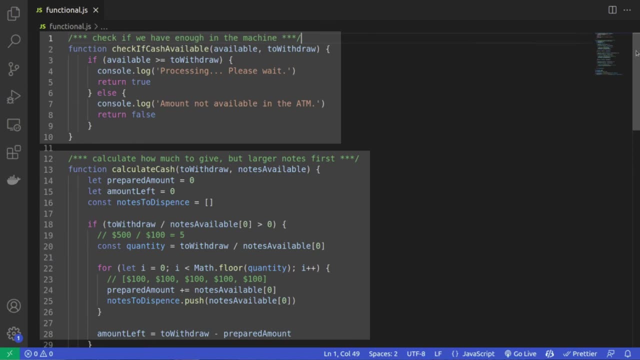 I tried rewriting the ATM logic in a functional way and now it looks something like this. As you can see, the logic is structured using pure functions that, ideally will have to return a value instead of mutating a value from outside. I haven't used any functional methods built into JS. 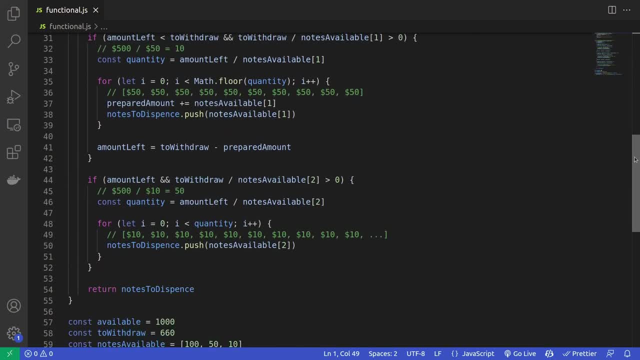 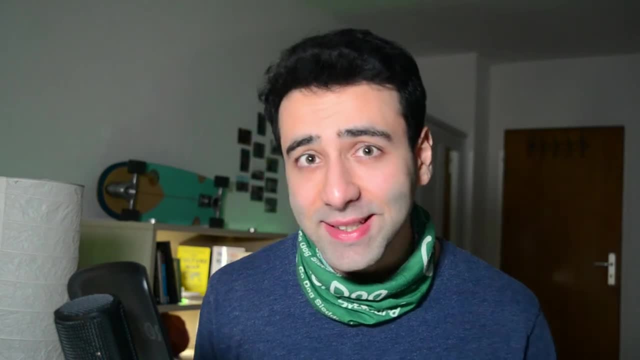 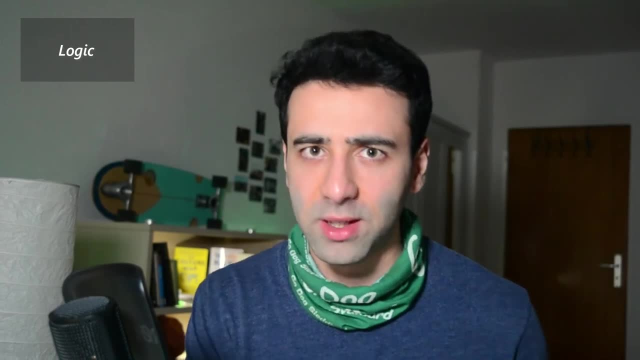 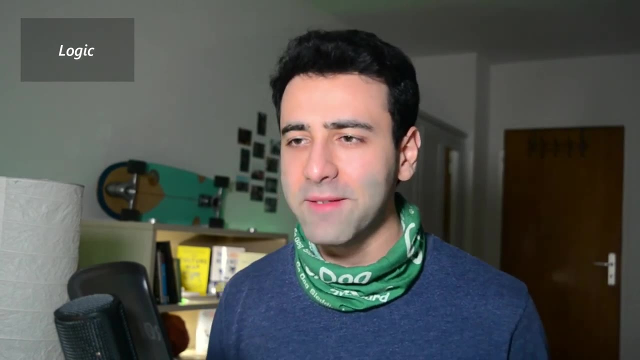 localization. We are going to start off by looking at the distribution of principles with such real physics guidelines, not as we've ever read about the word. Well, theителя Republic recommends to create a cultural base around the expression of human Vault. This is something very interesting. 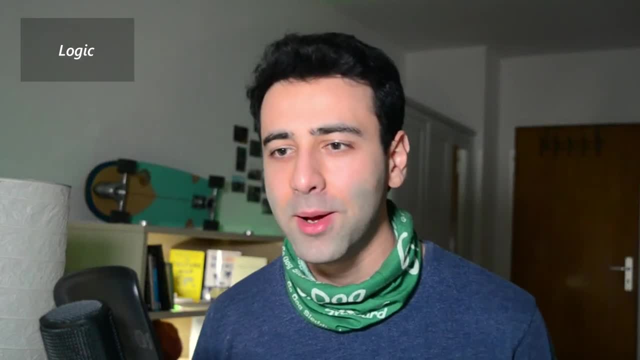 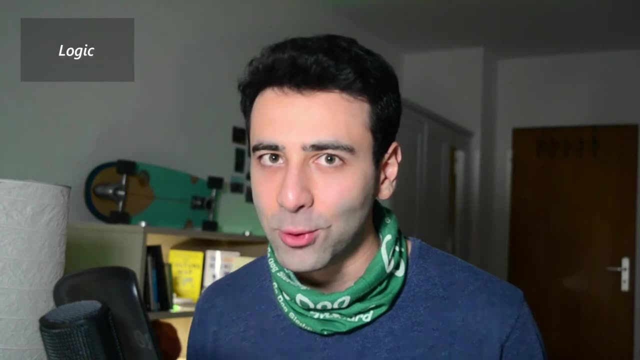 Many people already know that JONATHAN, please understand this. Mandalorian OK is dedicated mathematical statement. Programming languages such as Prolog and Mercury are specifically built for this. So let's actually take a look at a very interesting example: whether Socrates is mortal. 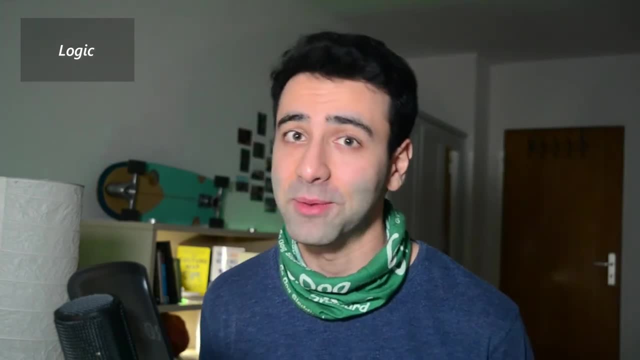 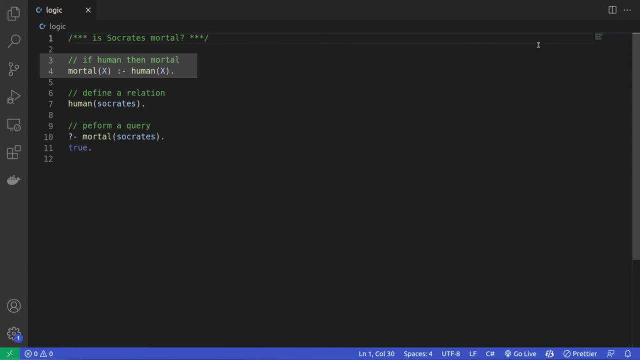 or not. using Prolog, We obviously cannot use JavaScript for this. So the first meaningful line here is interpreted as: if b, then a, meaning, if human, then mortal, aka all humans are mortal. The next line assumes that Socrates is a human. 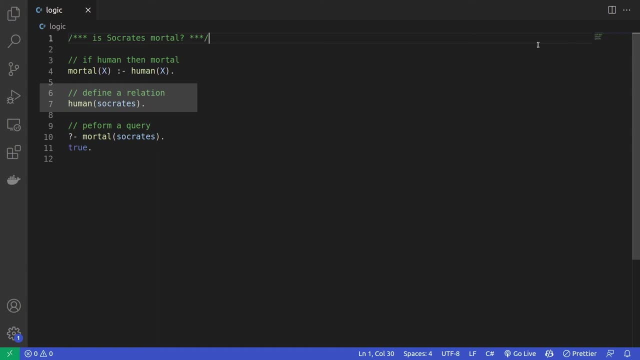 Cool, but how does that help? The reason we define these relations is that we can then perform queries. In this example we ask: is Socrates mortal? for which we get true, Because earlier we defined that if you're a human, then you are mortal too. 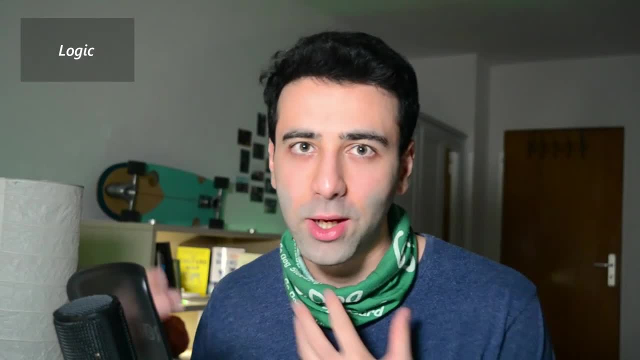 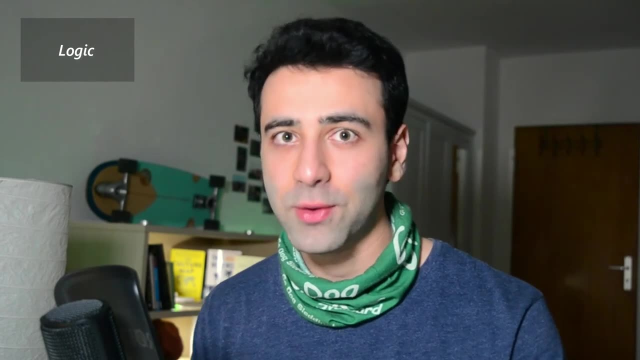 Logic programming is used for research and testing complex theorems and is closely connected to machine learning and AI. I'm gonna make a separate video on it, so make sure you're subscribed so that you don't miss it. Last but not least, data-driven programming. 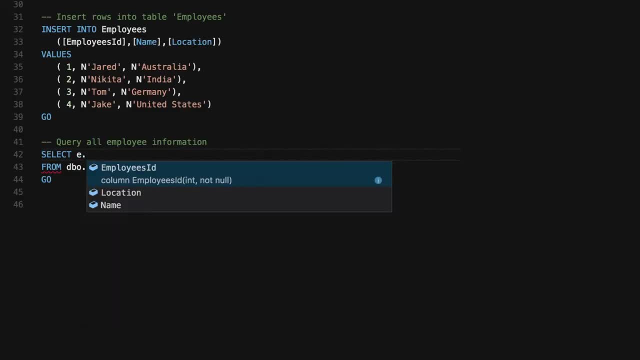 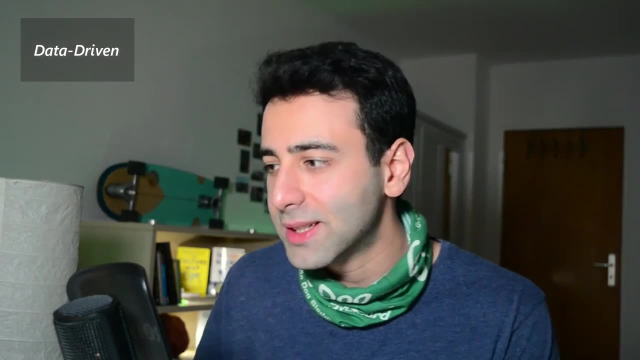 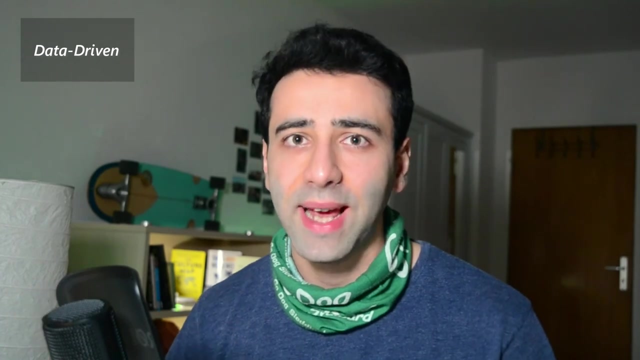 This one's pretty easy. Have you used SQL for dealing with relational databases before? I bet you have? Data-driven programming is exactly that. It's based all around data and its movement Statements are already defined by the database program that we can use to query, update and. 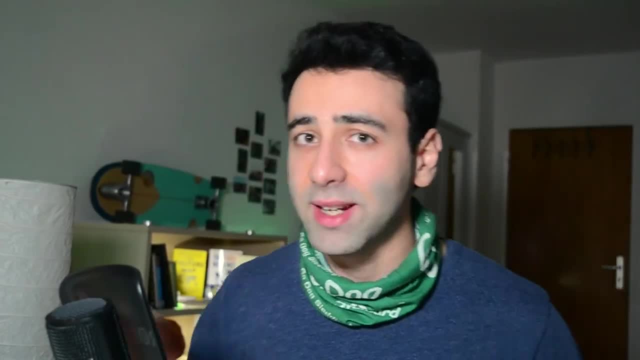 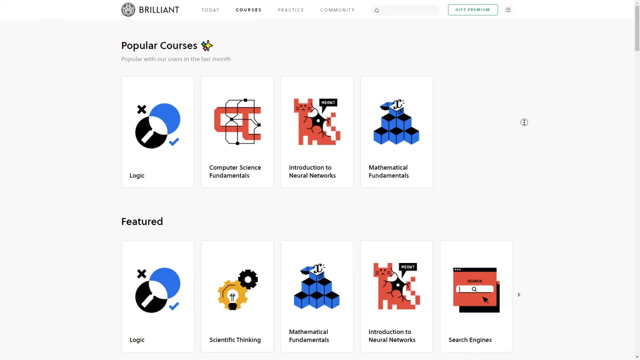 delete entities. Before we summarize everything with pros and cons, I would like to mention one of my favorite learning platforms that I use every day: Brilliant. Brilliantorg is an interactive platform where you can learn anything related to SQL, Anything related to STEM, science, technology, engineering and math.